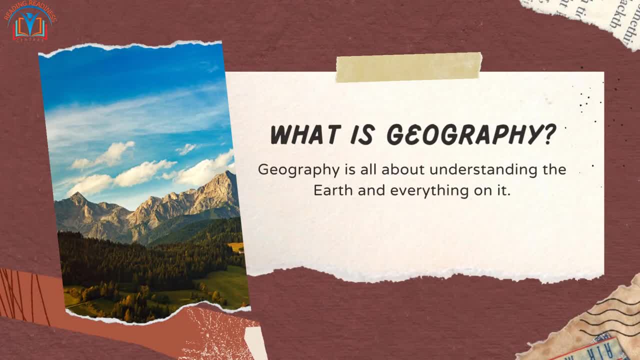 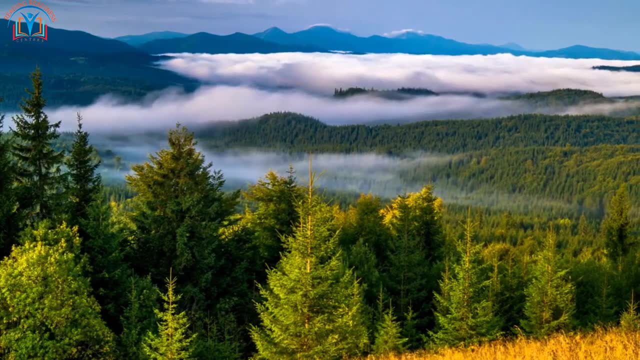 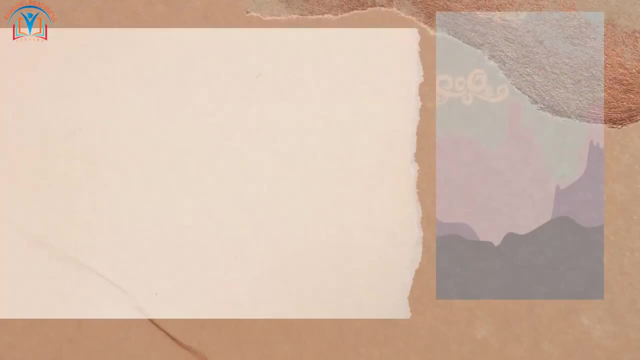 Geography is all about understanding the Earth and everything on it. Our planet is a big, beautiful place with so much to explore. We have mountains, rivers, oceans, forests, deserts and even cities with lots of people living in them. Mountains are gigantic landforms that reach high up into the sky. 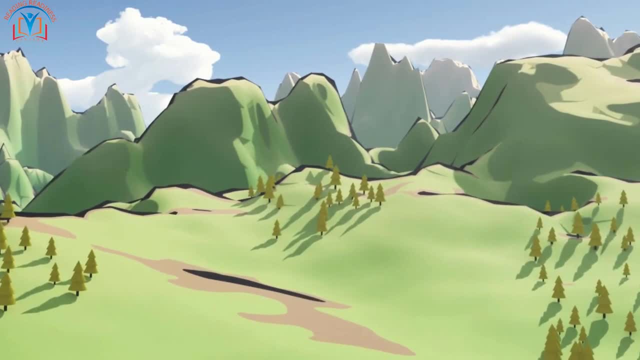